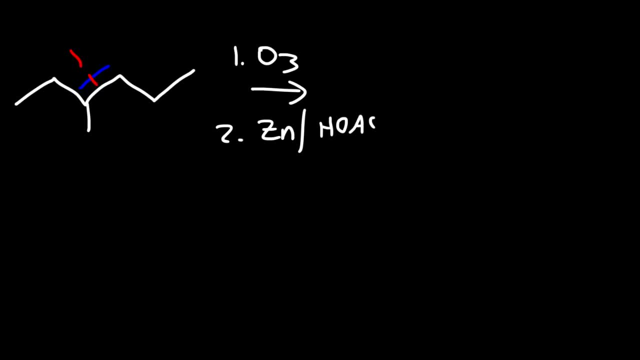 will have the same structure. So what's going to happen if we add ozonolysis and dimethyl sulfide? It's going to have the same effect. So I'm going to draw what I have left over after it's been split in two. So this is what I have, And now all I need to do is add an oxygen atom. So keep in mind. 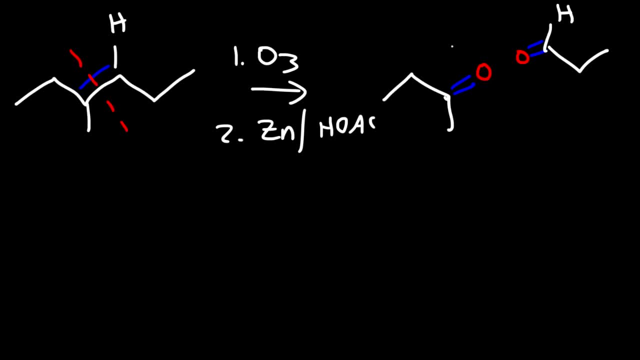 there's a hydrogen atom here, And so you can see that I have a ketone and an aldehyde After I split it. if this carbon is primary, it's going to be an aldehyde. If it's secondary, it's going to be a ketone, And so I can. 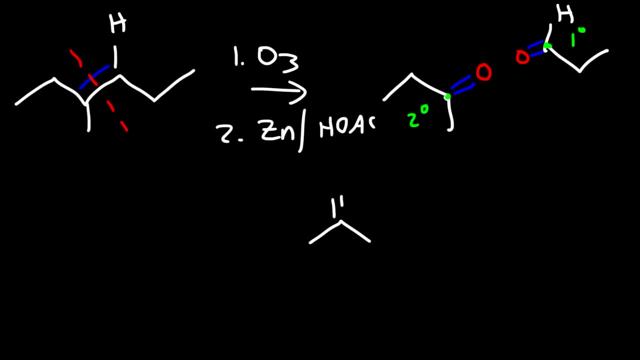 redraw the products like this if I want to. So I have two butanone and also propanol as my answers. So this time I got two different products. Now let's try some more examples. Go ahead and predict the major product of this reaction. 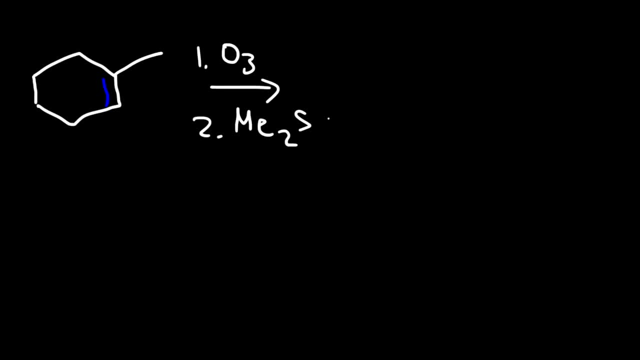 Dimethyl sulfide. you might see it like this: If you see ME, it's a methyl group. So once again, we're going to follow the same trend. So if you start with a ring, you're going to get a single molecule as opposed to two molecules. 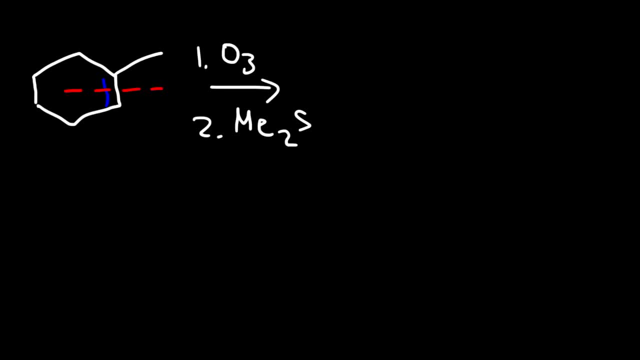 If you start with a chain, then you'll get two or more molecules per double bond. So we're going to draw everything the same way, but we're just going to break the double bond into two parts And then just add oxygen. So what we have here is a hydrogen, And so this is going to 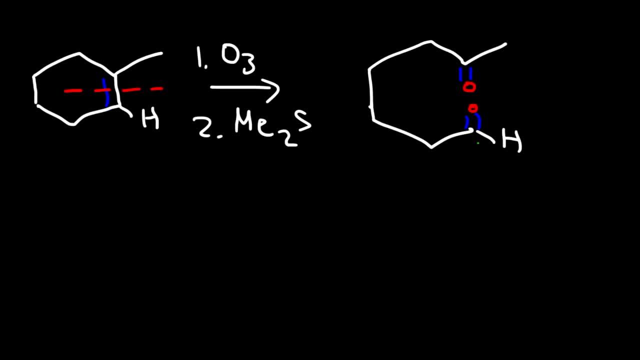 be a hydrogen. Now let's redraw this. So this is going to be carbon 1,, 2,, 3,, 4,, 5,, 6, and 7.. So let's start with the aldehyde function. We'll group that 1,, 2,, 3,, 4,, 5,, 6, 7.. On carbon 6, we have a ketone. 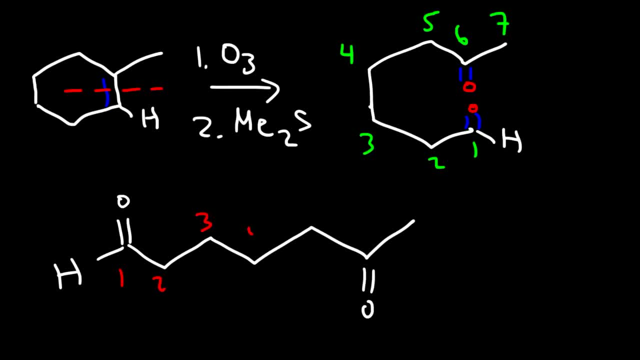 And so you can count it to make sure that we have the right answer. So this is the product for this reaction. That's all you need to do here. Now let's try another example. So go ahead and react this molecule With ozone followed by dimethyl sulfide. 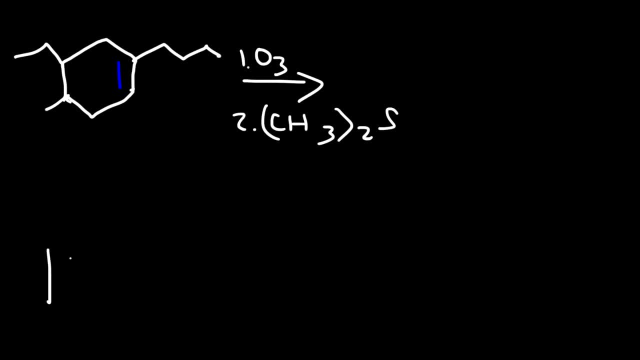 So go ahead and try. So I'm going to follow the same process as before, And that is by splitting the double bond into two parts And then adding an oxytratum to both parts, And so we have a hydrogen atom here. I'm going to put that here to indicate that. 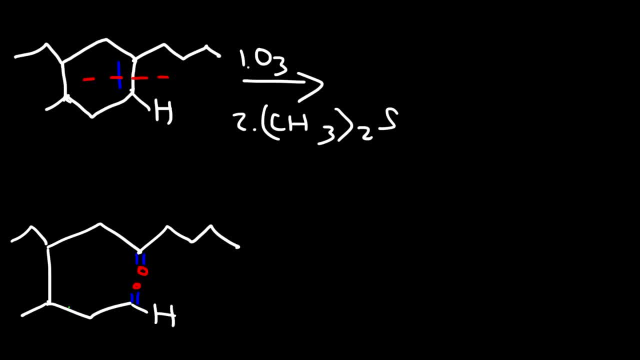 this is an aldehyde. Now let's count along this chain. So one, two, three, four, five, six, seven, eight, nine, ten, So we have 10 carbon atoms. Now we'll retry. This is 1,, 2,, 3,, 4,, 5,, 6,, 7,, 8,, 9,, 10.. 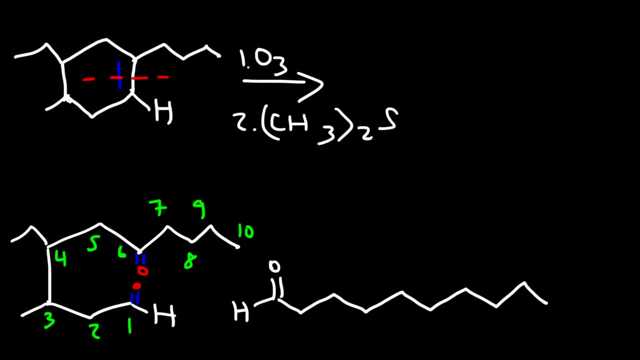 Now, Now, attached to carbon-3, there's a methyl, and then there's an ethyl. on 4, and on 6, we have a carbonyl group. And just to make sure we did it right, this is 1,, 2,, 3,, 4,, 5,, 6, and so forth. 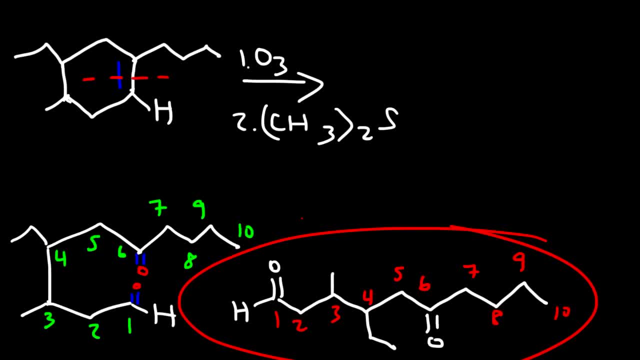 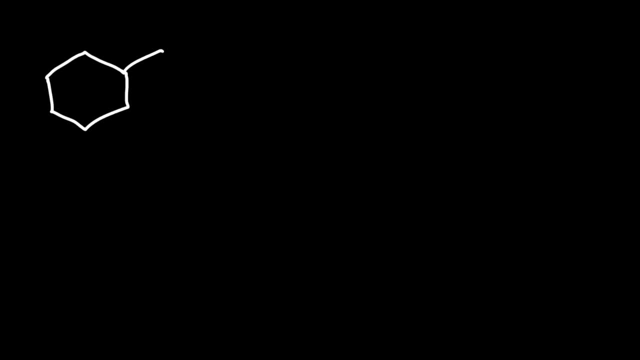 And so this is the product of the reaction. Now let's try another example. So let's say we have a double bond here and another one here and here as well. So let's use ozone again, And this time let's use zinc and acetic acid. 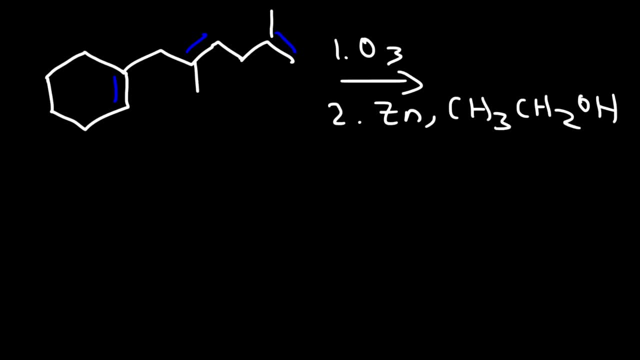 Go ahead and predict all the products that can be formed in this reaction. So every Everywhere we see a double bond. we need to split it into two parts. Now, keep in mind there's two hydrogens on this carbon atom, and there's a hydrogen here and another one here. 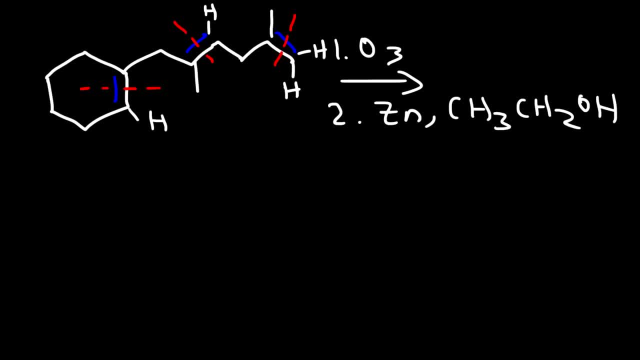 It's always good to place those hydrogen atoms to tell if you're going to get an aldehyde or a ketone. So let's begin. So let's start with the ring. So we're going to have two oxygen atoms there and then we have another double bond in this region. 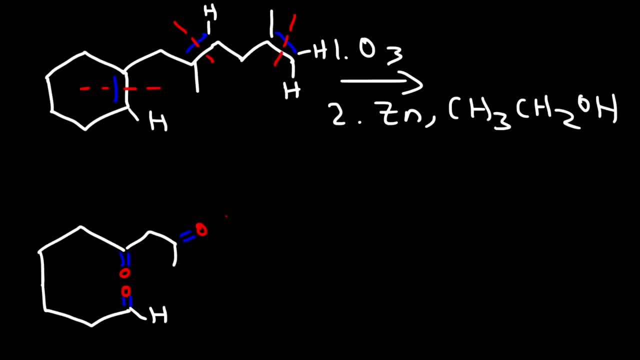 And so that's going to be a ketone, And here we have a hydrogen- some at this point right now, or this area- And then there's another double bond here And then we have another oxygen facing that ketone. And so these are the three products that we have. 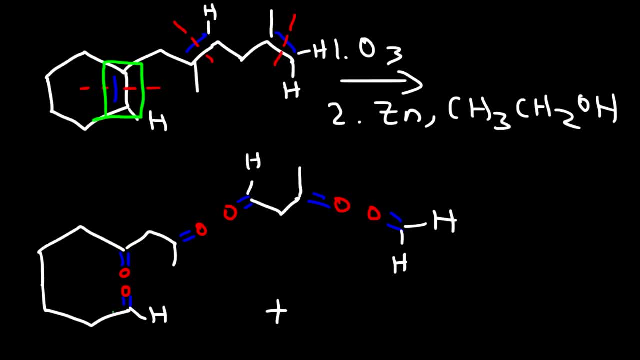 So everywhere there's a double bond. all I did was I split it into two carbonyl groups, And so here We have an aldehyde and a ketone. You can see that, And in this area we also have another aldehyde and a ketone. 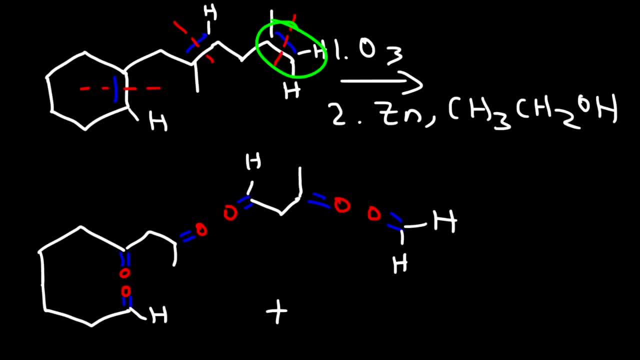 So these are the products of this reaction, And then you can redraw it if you want to. So let's go ahead and do that. So the first product is simply formaldehyde, Which looks like this, And then the second product has: It has four carbon atoms. 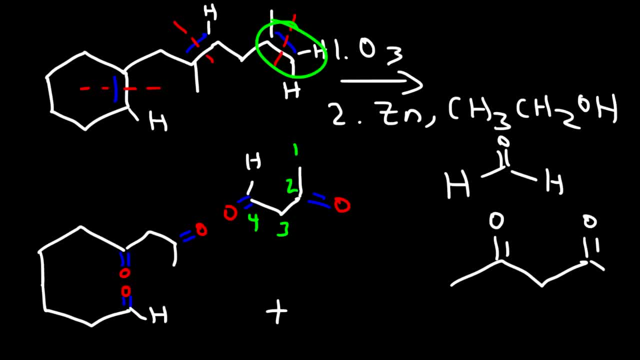 So we have a ketone and an aldehyde. Now let's redraw this molecule. So I'm going to start with the aldehyde again. So this is carbon 1, 2, 3, 4.. 5, 6,, 7,, 8, 9.. 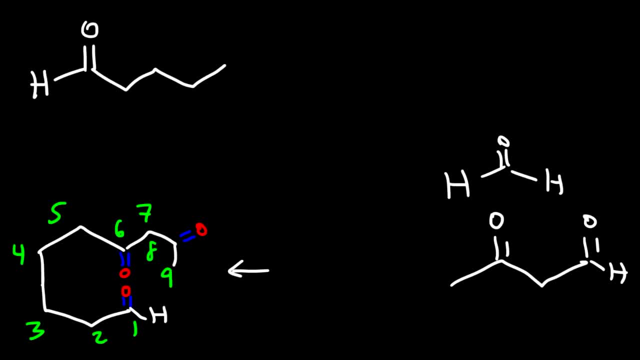 So that's the first carbon, Second, third, fourth, fifth, sixth. On carbon 6, we have a ketone, And then 7,, 8,, 9.. On carbon 9, we have a ketone. So it's always good to double check to make sure that you counted it right. 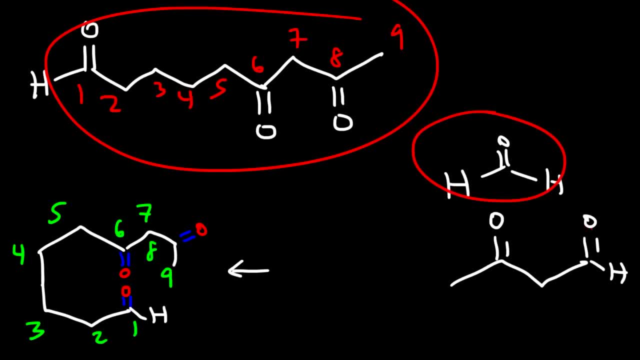 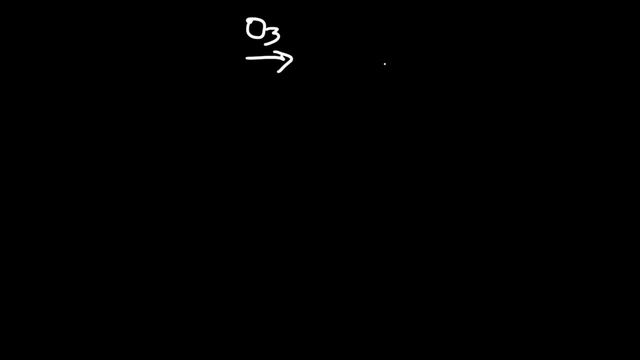 And so these are the three products of this reaction. Now, what if you're given the products of the reaction? So let's say we have a ketone and an aldehyde, How can we determine the original alkene that made those two products? 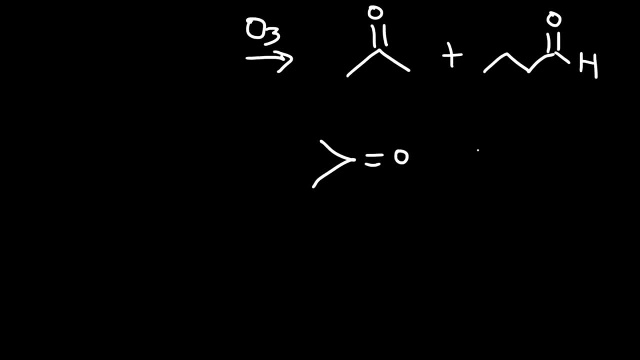 So what I like to do is draw the carbonyl groups facing each other And then simply just connect them. See, what you want to do is get rid of the two oxygen atoms and connect the two molecules by means of an alkene. 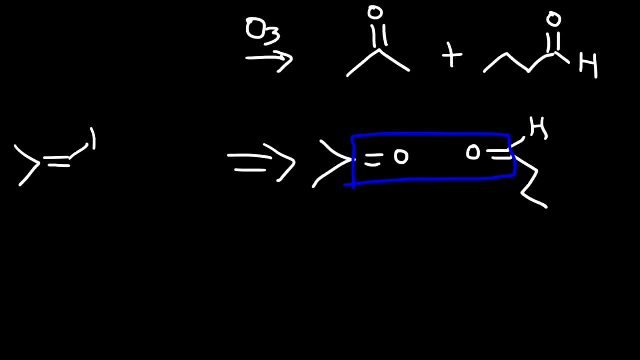 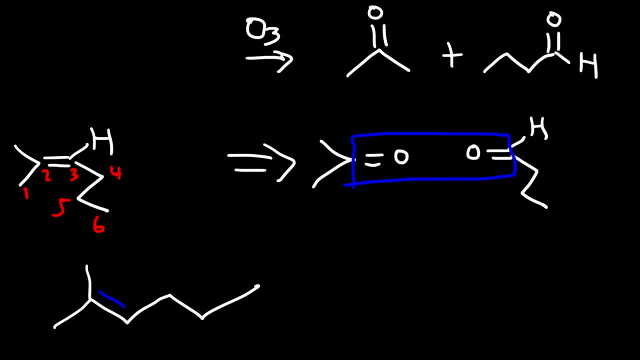 And so we have 2-methyl 2-hexene as our starting material, And so that's how you could find the original alkene that was used to make these two products. For the sake of practice, let's try a similar example. 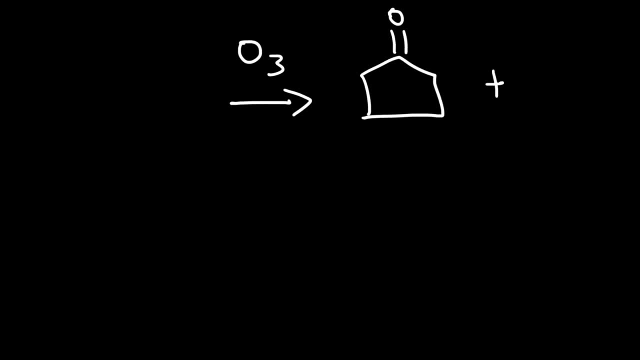 So go ahead and draw the alkene that was used to make these two products. So let's follow the same process. Let's begin by drawing these two molecules. Let's begin by drawing these two molecules in such a way that the carbonyl groups are facing each other. 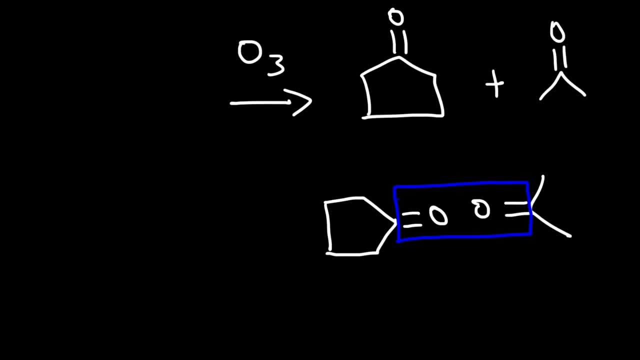 And then replace what you see here with an alkene, And so the starting material looks like this, And that's all we need to do, And so that is the alkene that was used to make these two compounds. So let's try one more example.